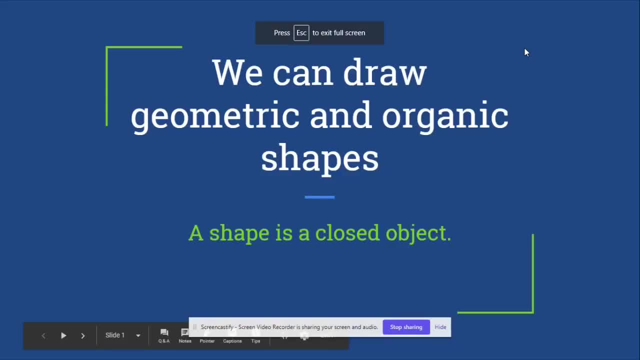 Hello, today we're going to talk about geometric and organic shapes. So we learned back in first grade and kindergarten that a shape is a closed object. So there's a difference between shapes and lines. Your line has to connect to make it a shape. Now we're going to learn how we can group. 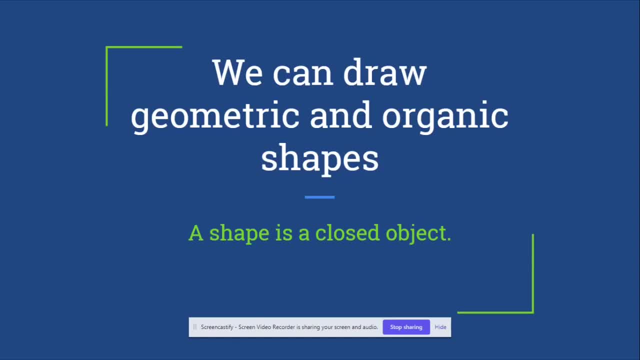 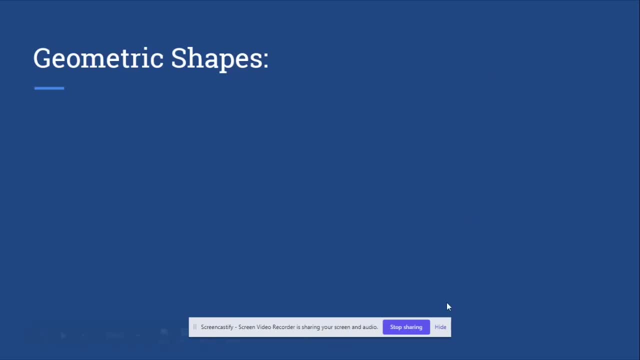 shapes into two different families: geometric shapes and organic shapes. So geometric shapes are shapes that have a name. They're shapes that we talk about in math a lot and you will recognize these shapes because we've been talking about these since kindergarten. So geometric shapes. 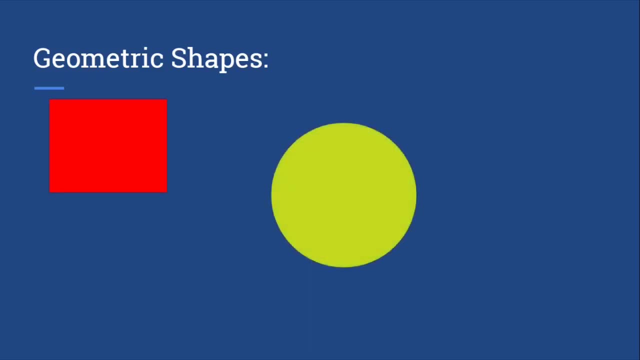 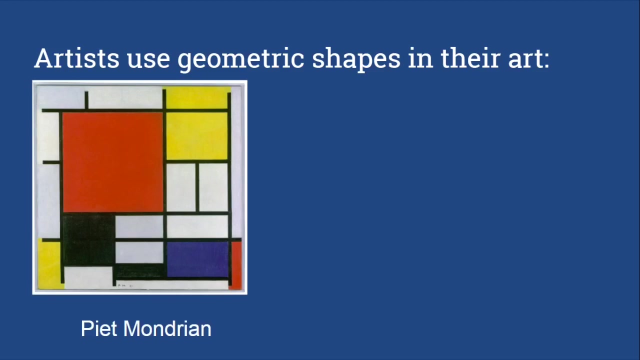 are shapes like square, circle, triangle, diamond, heart circle. Artists use geometric shapes in their art all the time, So see if you can find the geometric shapes in this painting by an artist named PA Mondrian. Let's take a second to pause. 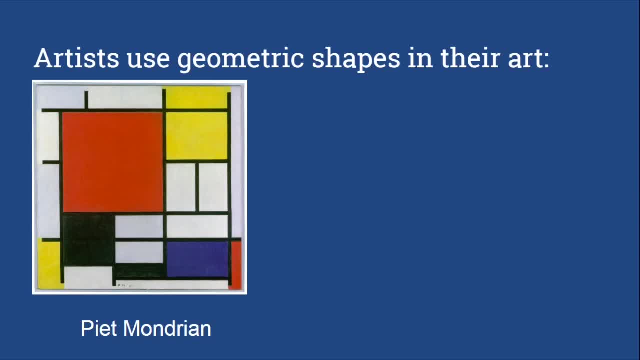 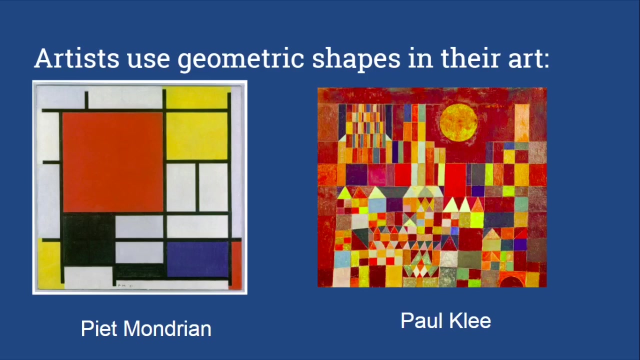 the video and look at the geometric shapes here. So as a bonus question: what color family do you see in this painting? also, Here is another artist that uses geometric shapes in his artwork: Paul Clay. We can find geometric shapes in this painting. Let's see if you can find them, Turn and share with your neighbor. 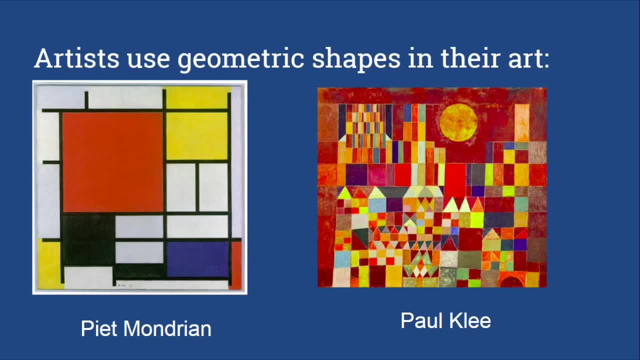 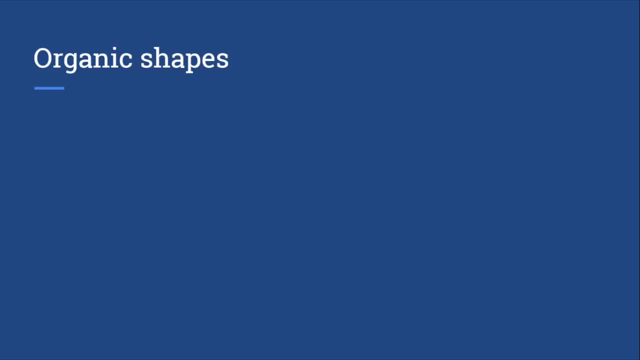 So the opposite of geometric shapes is organic shapes. Organic shapes are shapes that we see in nature. They're natural shapes, free-form shapes. We've seen them in art before. They're shapes that usually don't have a name. Sometimes they have. 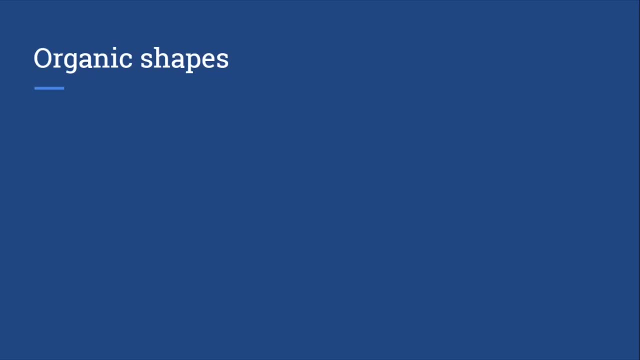 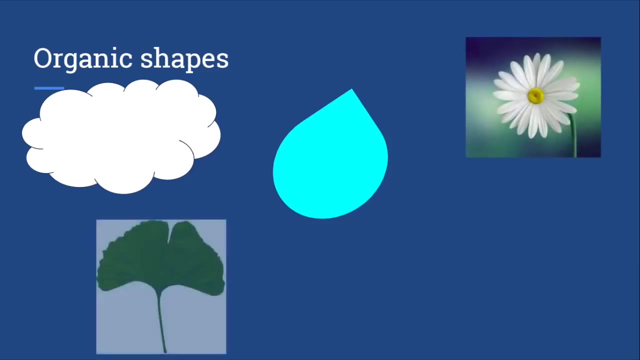 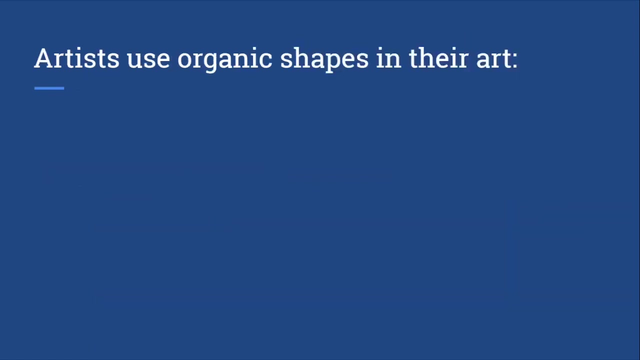 a name, but sometimes they don't. They are the opposite of geometric shapes, So you won't often see flat sides on organic shapes. So shapes like clouds, rain drops, flowers, leaves and free-form shapes like we see here, those are all organic shapes. Artists use organic shapes to paint. They're.